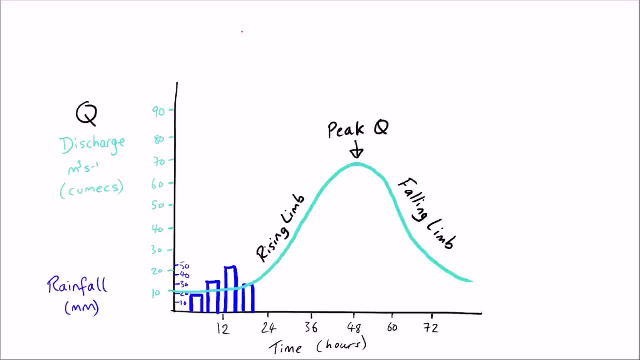 symbol of discharge, so we're going to be using that in this presentation. You can see here how full the river can get and in some cases it's cases it actually overflows its banks. You might see a little line on your stormwater graph indicating the bank full discharge and this would be when the river gets right to. 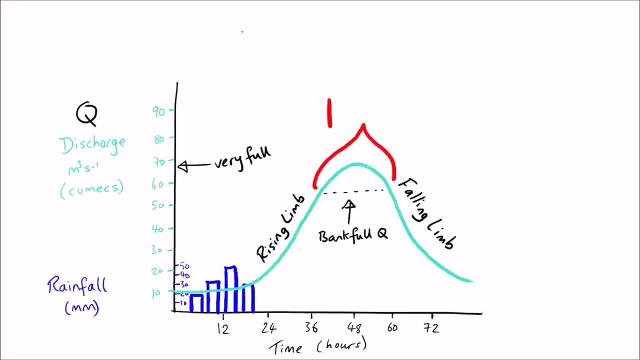 the top, and if it goes beyond that line, it means there's a flood. Now it's really important that we learn all these key words and phrases, so what I'm going to do is write a list at the side so we won't forget them. 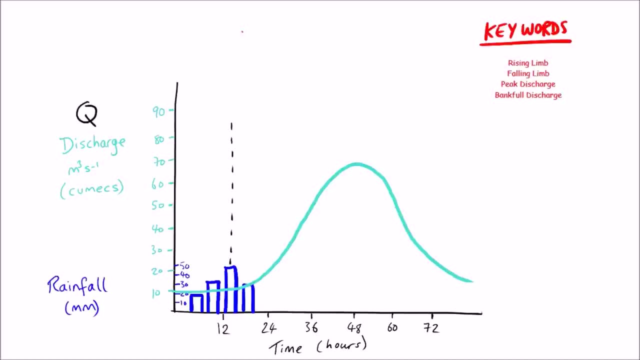 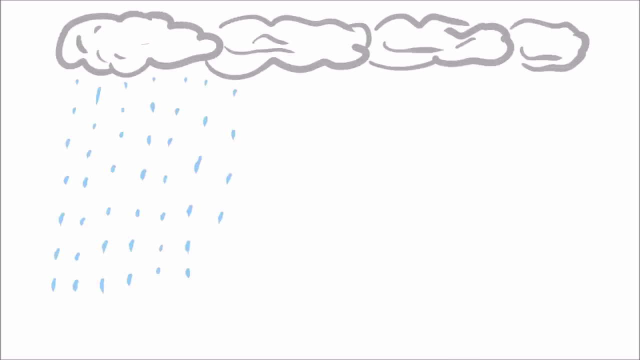 Another really important key term and concept of the stormwater graph is the lag time, and that is the gap between the peak rainfall and the peak discharge. So why is there a delay? Let's take a look. Here's some rain. Here's some rain. 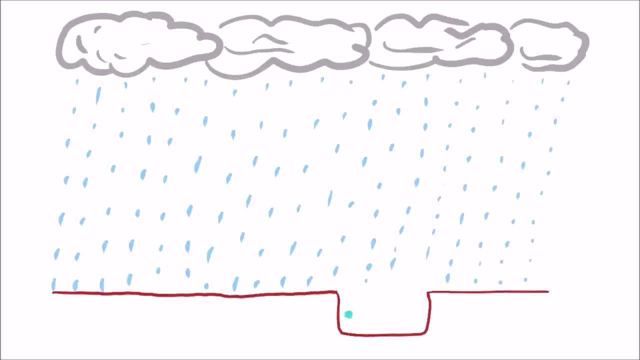 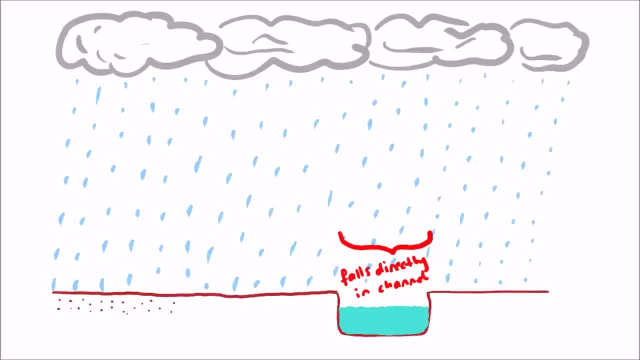 channel itself. so it wouldn't make sense if the river level suddenly rose instantly as soon as it started raining. Most of the rainfall actually reaches the river via other processes which you would have learnt about when you did the drainage basin hydrological cycle When it first started. 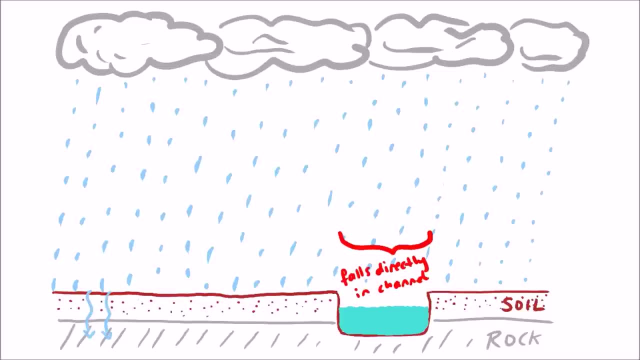 when it starts raining, the water will infiltrate the soil and, assuming it's permeable, it will percolate down into the rock below. This is called groundwater flow or base flow, and it's the slowest transfer out of the ones we're going to be talking about. 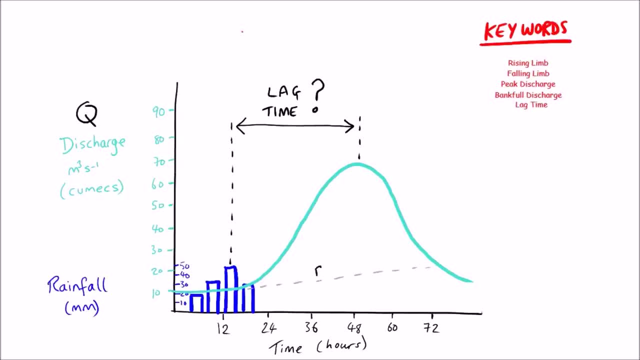 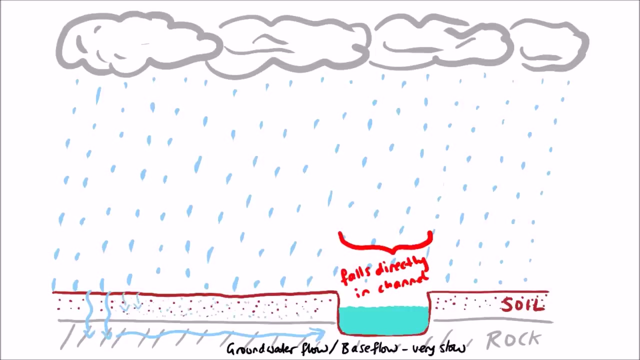 So let's draw it onto the graph. This part here going up very slowly is the base flow And you can see that it keeps rising, keeps adding water to the river long after it's stopped raining. As the rain keeps falling, the soil will start to fill up with water and become saturated. 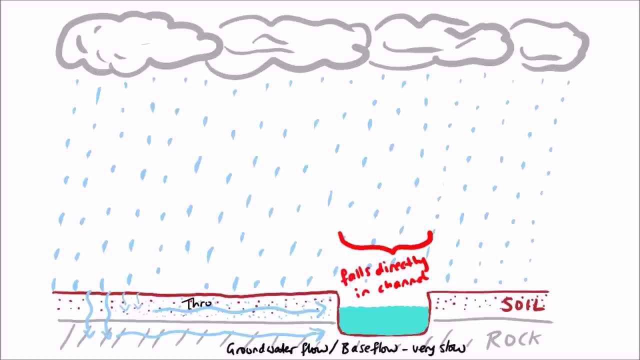 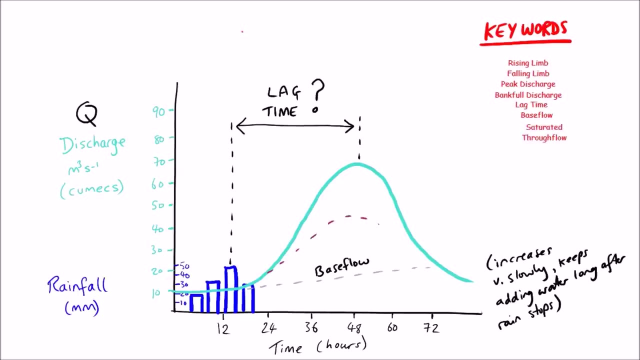 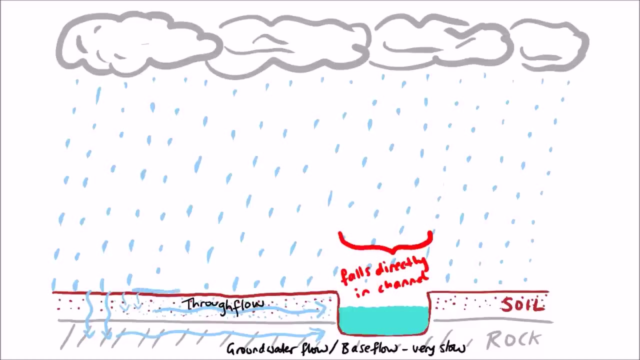 particularly if groundwater stores become full or if the rock is impermeable. The water will then reach the river via through flow. So let's just add that onto our graph here and you can see this is faster than the groundwater or base flow. Finally, the third way that water can reach a river in a drainage basin is if surface. 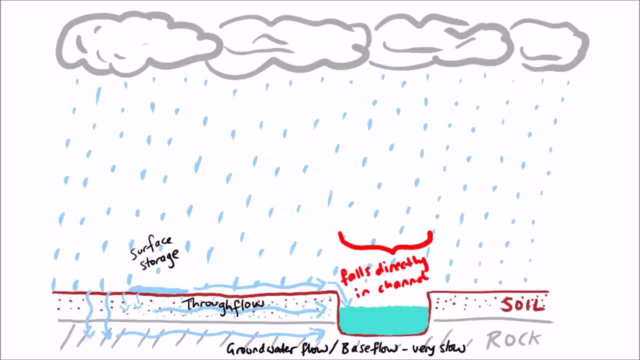 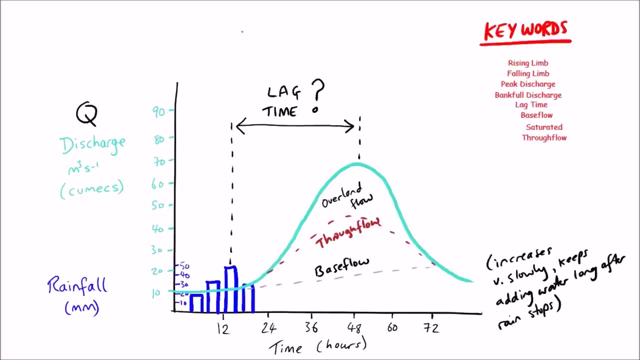 storage builds up and then flows over the ground as overland flow. This process is much faster than the other two, and this is the one that can often lead to flooding, particularly in urbanised areas. So let's add this final component onto our graph and add a few more keywords here at 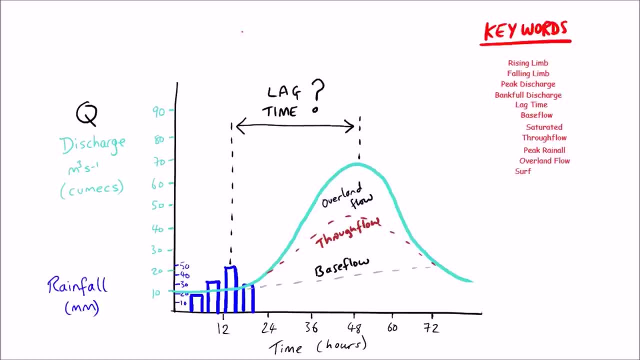 the side. Apologies, I forgot to mention peak rainfall. Peak rainfall is when the rainfall reaches its maximum and where you measure lag time from. Okay, so now we know what a storm hydrograph is. we get to the really interesting part. 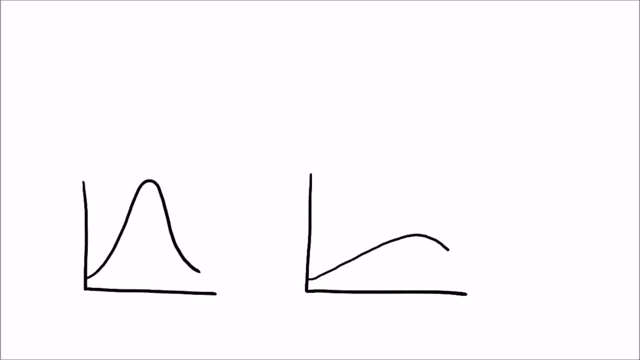 which is the different shapes that a hydrograph can take. Now you can see, the one on the left can be described as a flashy hydrograph, whereas the one on the right is delayed. Flashy hydrographs are characterised by a very high peak and it's very steep, very steep and 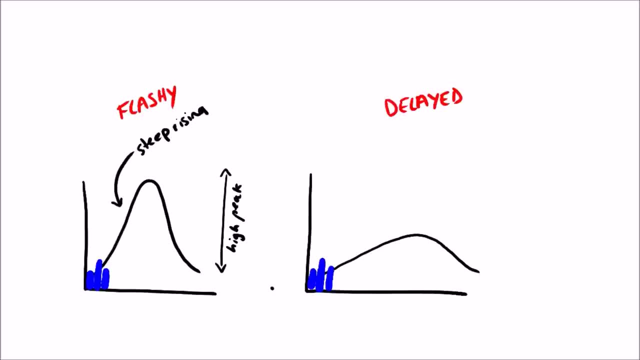 rising and falling limbs, Whereas delayed hydrographs tend to have a long lag time, a lower peak and a much shallower curve overall. Let's add these words to our list as well. So why do these hydrographs have different shapes? Well, hopefully it's obvious to you. 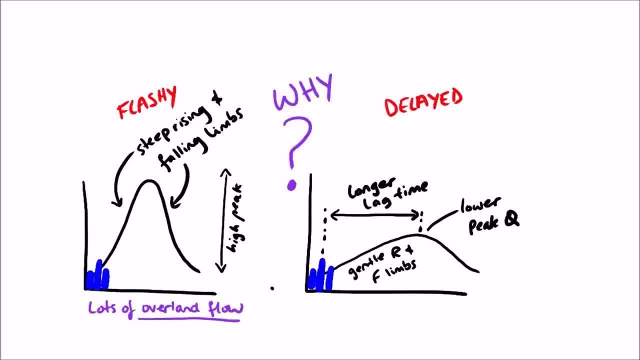 by now that the one on the left will have lots of overland flow, whereas the one on the right will have mostly throughflow and base or groundwater flow. Now, I'm not going to go into a great amount of detail about why this is, but hopefully 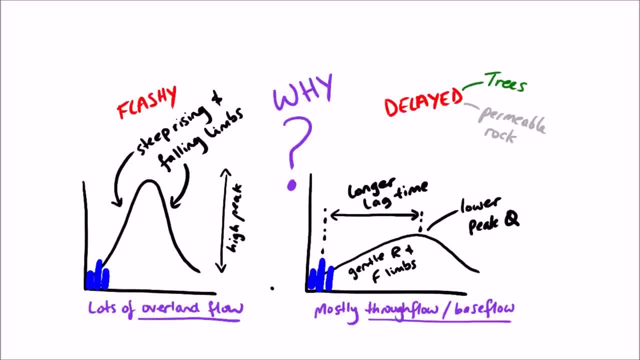 you know from studying the hydrological cycle that drainage basins with flat land, lots of trees and permeable rock, We'll have much slower transfers than areas with urban surfaces, steep slopes, places that have impermeable bedrock underneath the soil and possibly have very thin soil. that 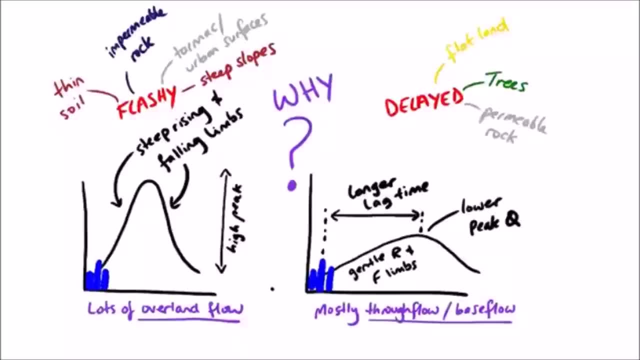 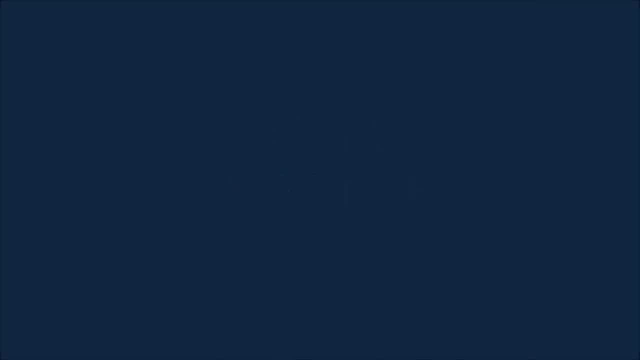 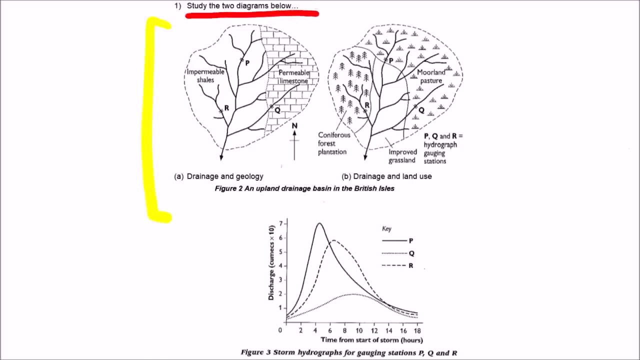 can be easily saturated. Okay, so let's take a look at some exam questions. Now. the first thing you have to do, as with any question in the exam, is make sure you read every word very carefully so you know exactly what the question is asking you to. 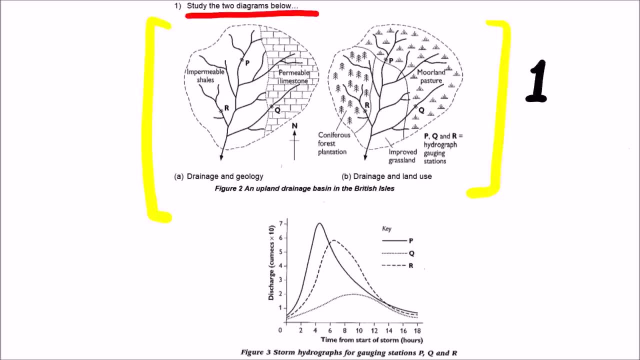 do This particular question. it contains two figures. Okay, the first one has two drainage basins, So let's have a look. We've got drainage and geology on the left, so that shows the rivers and the type of bedrock. 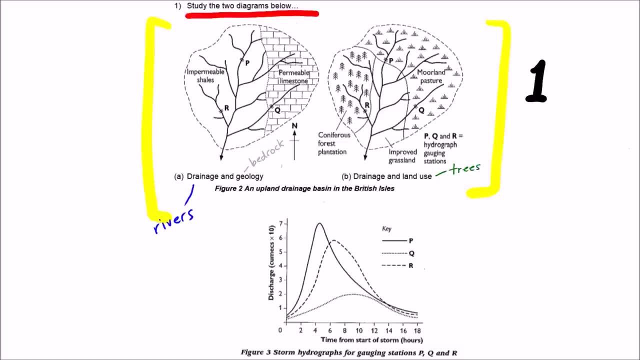 underlying, and then B shows the drainage. again it shows the rivers, but also the land use this time. So are there trees recently? So are there trees, for example, Is it bare ground? It could be arable farming, it could be grassland. 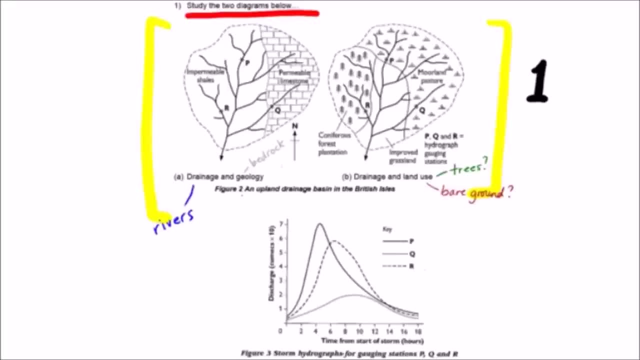 All of these things are going to affect how the river responds when it rains. Now make sure you read the figure labels, okay? As you can see, this is an upland drainage basin in the British Isles. I can't tell you how many people got this wrong and thought that it was two separate. 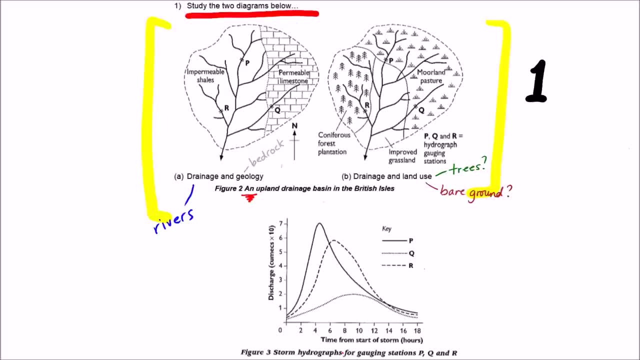 drainage basins and lost a lot of marks because of it. So just a clarification. So just to clarify that figure two shows two different characteristics of the same drainage basin. okay, One shows rock, the other shows land use, but it's the same set of rivers each time. 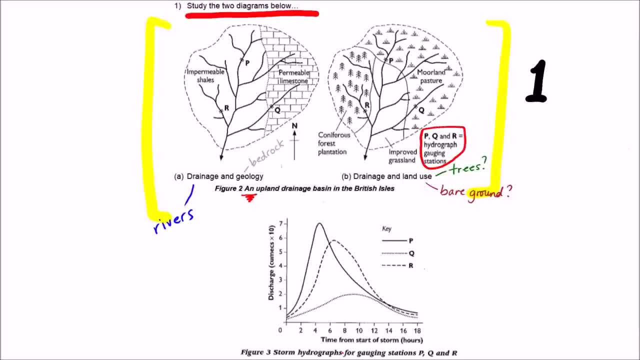 Now the next thing to notice is the three hydrograph gauging stations: P, Q and R. This is where discharge is measured. This is what links the first set of diagrams to the second one. So this is the hydrograph, or figure three, which, if you read at the bottom, is dorm. 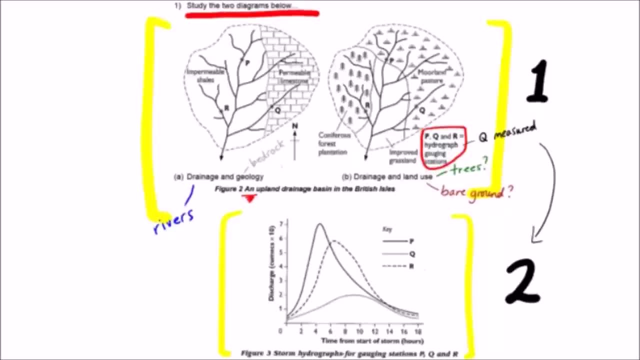 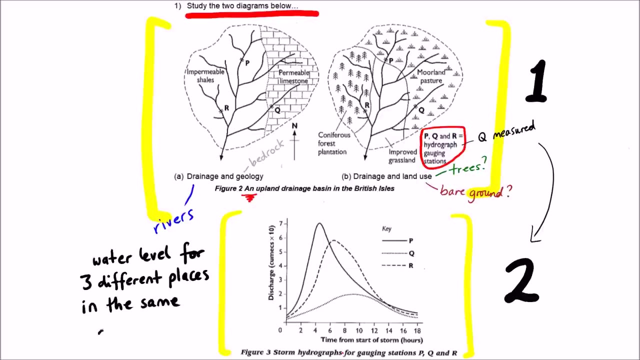 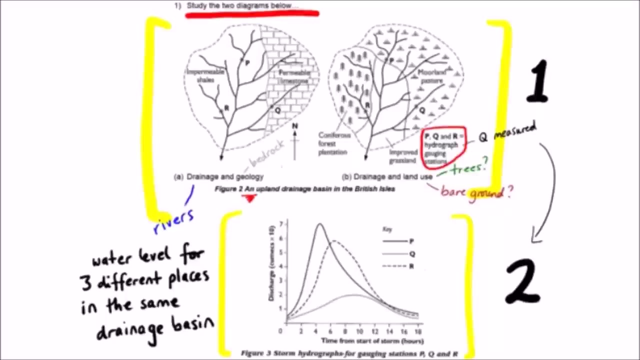 hydrographs for the three gauging stations P, Q and R. So it basically shows the water level for three different places in the same drainage basin. It is not three different drainage basins but you can see from the map above that they're. 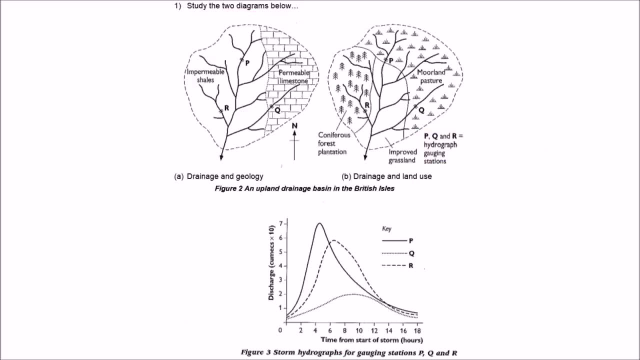 all in the same one. Okay, Now for the first question. you have to compare the dorm hydrographs for stations P, Q and R, as shown on figure three. This is worth five marks. This means that it's level marked okay. 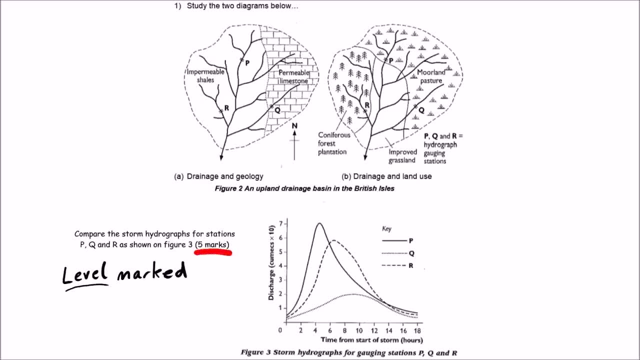 Remember the questions that are four marks and below are point marked, but if it's five and above you can't just write five points and get five marks. but it's marked in two levels. So to get to level two you need to have a high level of sophistication, high level. 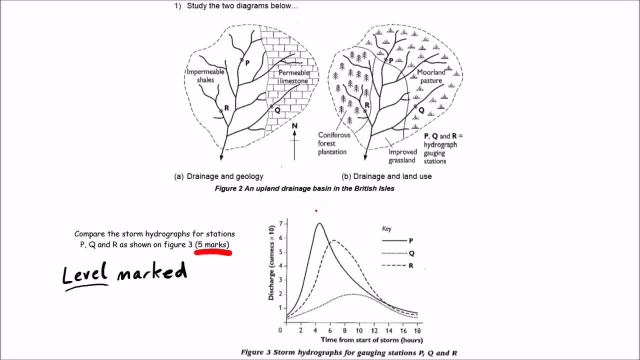 of understanding. So how can we do this Before we answer? one thing that I find really helpful with graphs like this is to colour code them. So I'm just going to put here P in red, and then we'll put Q, which is second, but it's. 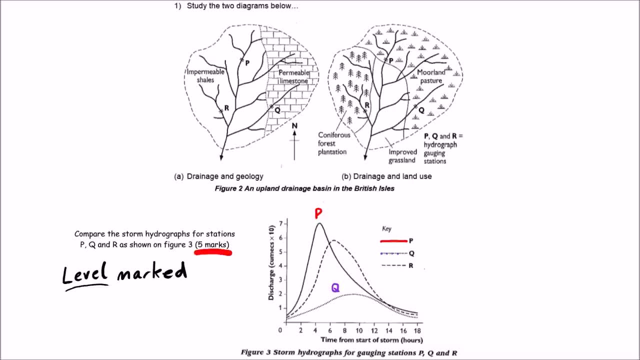 actually bottom on the graph, which is why it's so confusing. We'll put that one in purple and then I'll put R in green. okay, A lot of people get confused between R and Q because they're the different way round. 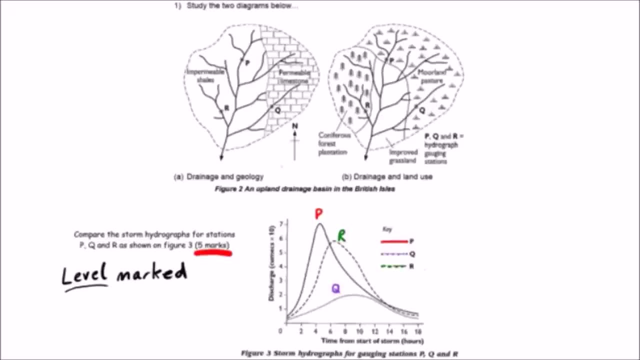 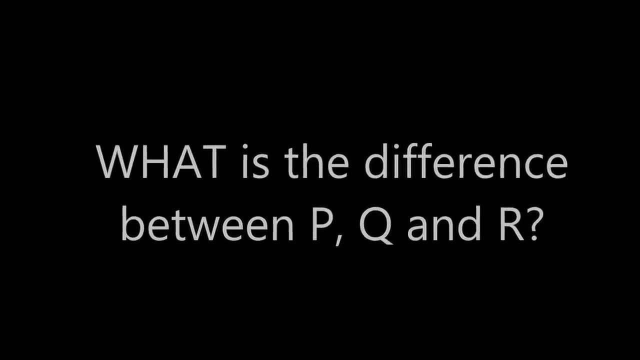 of the key, So make sure you don't fall into that trap. Now all you have to do for this question is to say how P, Q and R are different from each other. You don't need to explain why they're different. 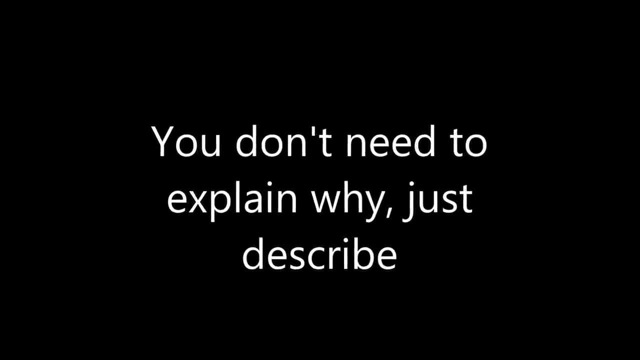 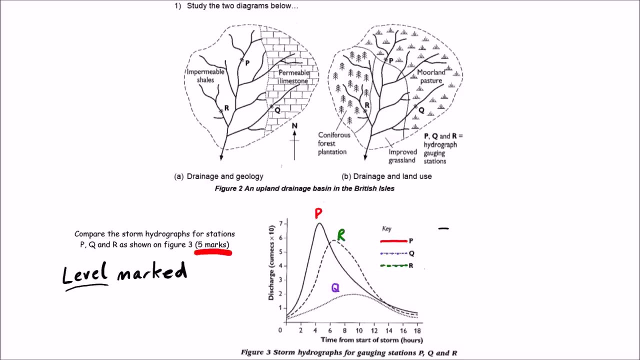 You just need to describe the graphs, okay, So don't try and put in any explanation. If you're not sure about this, just look ahead to the next question and you'll see why. So, to get up to level two, the first thing you should try to do is use key words. 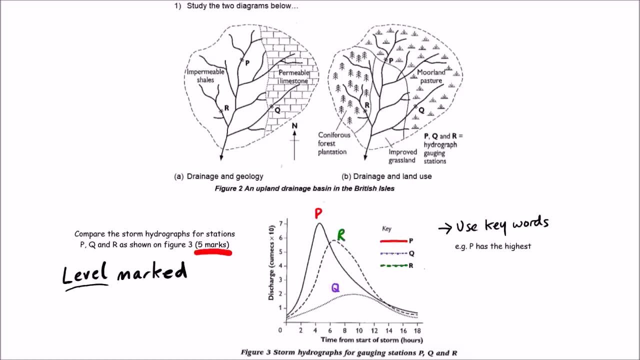 So example: Instead of saying that P has the highest water level, you might say that it has the highest peak discharge and use that key phrase. Secondly, you must obey the command word of the question. So in this case it says to compare. 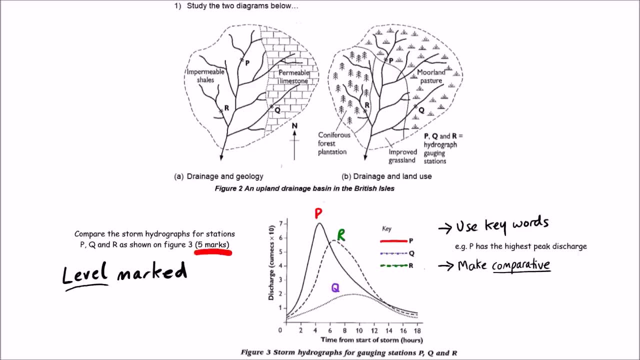 Therefore, you should try to use comparative statements in your answer. You can do this actively by using words such as whereas, conversely or however. Next, if you're given a graph in any question, you should always use the key phrase. 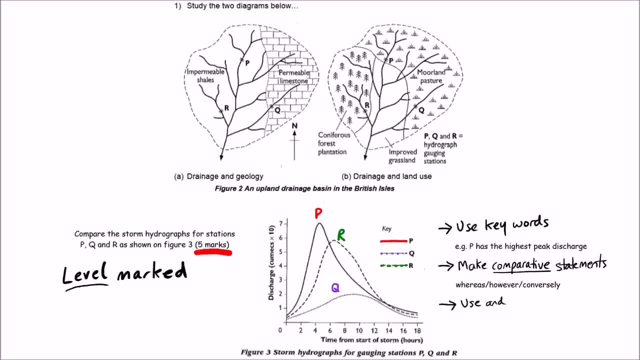 If you're given a graph in any question, you should always try to use and even manipulate the data from the graph. If they give you a graph with numbers, they'd like you to use the numbers and even to do basic calculations with them in your answer to show your understanding. 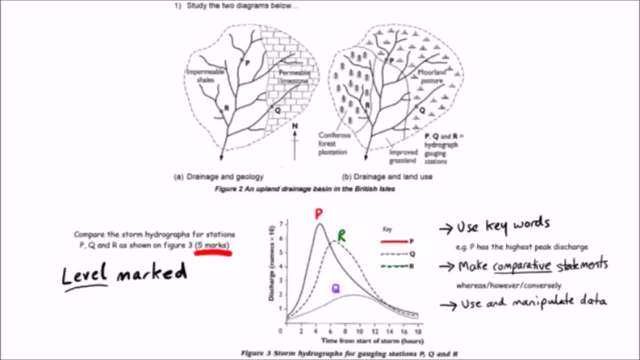 So, for example, P has the highest peak discharge would be a level one statement. In order to make it a level two statement, you could add of 72 max. okay, So you see, you're adding that little bit more detail and that's the sort of thing. 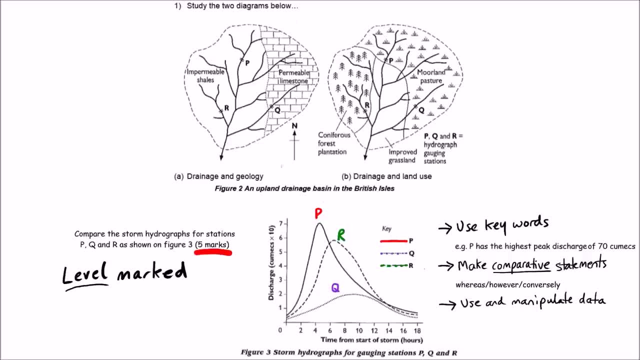 that can push you up to the next level. Now, to give you an example of data manipulation, you could say that Q peaks at only 21 cumecs, more than three times lower, or less than a third, that of station P. 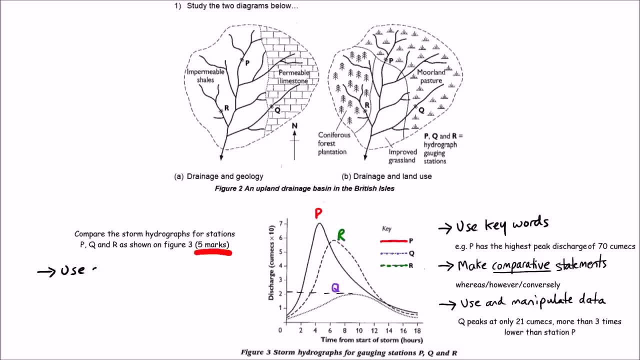 When you do read numbers off a graph, make sure that you use a ruler, as the mark scheme can be really picky about accuracy. Finally, you must refer to all three lines on the graph to get to level two. The next thing you have to do is to suggest reasons. 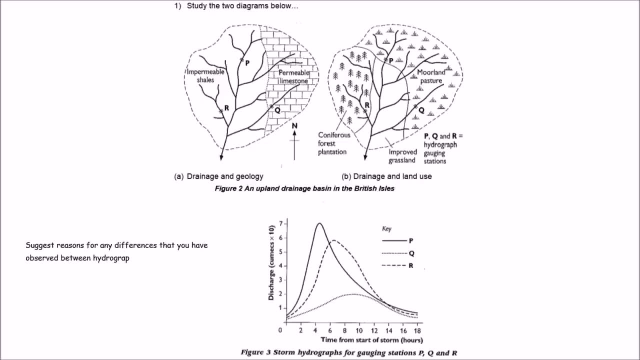 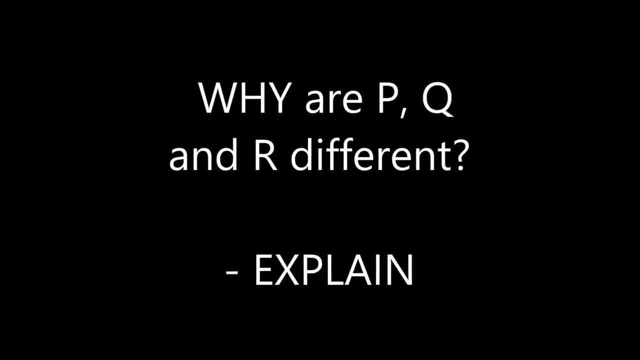 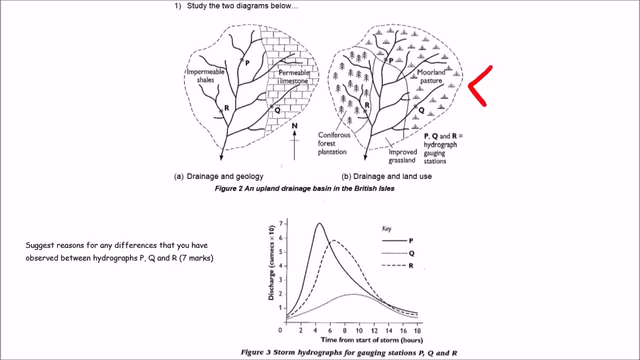 For any differences that you have observed between hydrographs P, Q and R. In other words, now you have to say why, you have to explain why they are different from each other. Now this question is a bit more difficult because it requires you to link the two diagrams together. 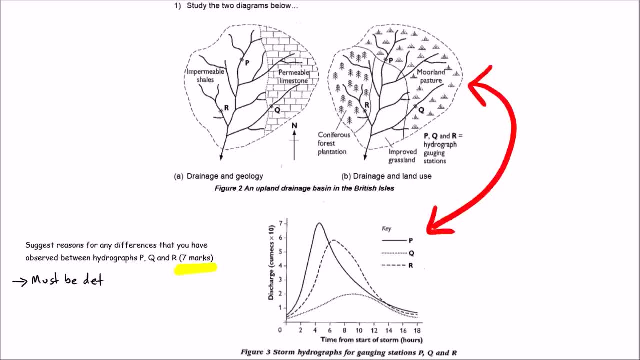 It's worth seven marks so it must be detailed. You must use T words in your answer, so use the list that we did at the beginning. You could structure your answer by looking at geology first and then land use, So try to make that structure really clear in your answer. 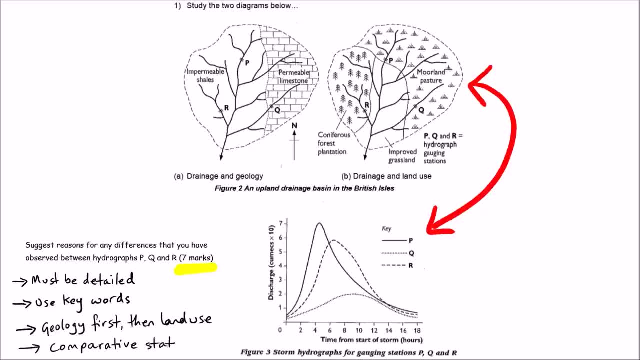 And again you must use comparative statements, because the question is asking you about differences. Now you must use the diagram, okay, So don't suggest any reasons that are not obvious from the diagram. Don't start talking about, for example, steep slopes. 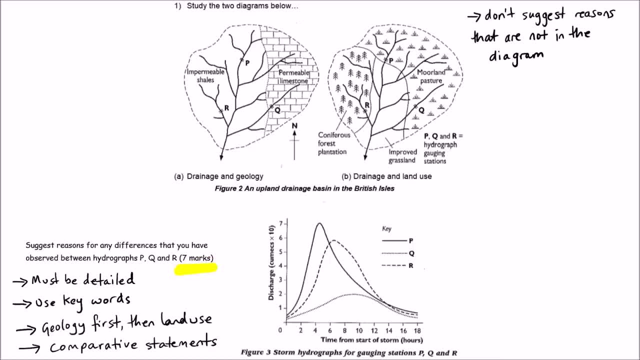 or urbanisation. I'm just going to label my hydrographs again to make it clear when I answer, And then we'll have a look at some example answers. So number one, P, is higher than R, Which is right because it is high up and must have steep slopes. 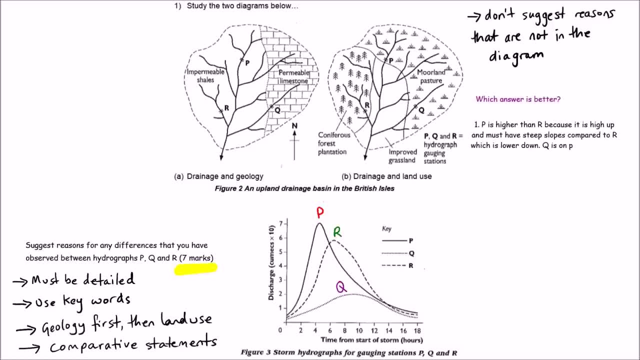 Compared to R, which is lower down. Q is on permeable rock so the rain can soak in. R has lots of trees that absorb all the water, But Q has moorland, which absorbs less water. Finally, at R, the water can't soak into the ground. 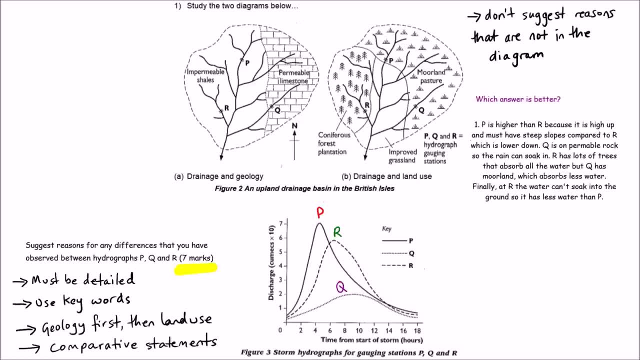 So it has less water than P. The first thing I would say about this answer is that you can't tell on the diagram that there's any steep slopes, Okay, so don't make stuff up. Secondly, there's really missing opportunity. 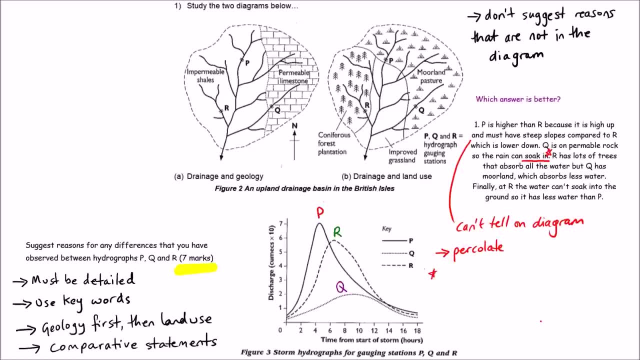 To use key words. they've said soak in, but they could have said percolate. And then they haven't developed this point. Okay, they haven't linked it to the hydrograph. They haven't said what impact the fact that it's impermeable will have. 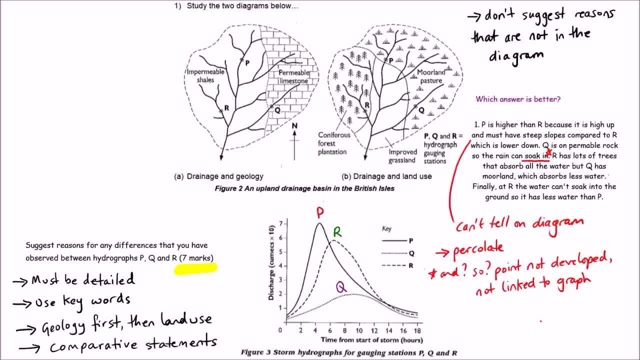 On the shape of the hydrograph. They've made the same mistake in the next sentence And overall their answer doesn't really have much structure. It's not very clear And there's definitely not enough detail to get seven marks. So let's have a look at another answer. 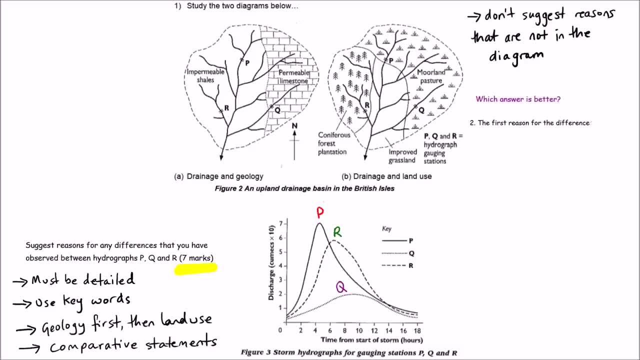 This student has said. The first reason for the differences is that P and R are on impermeable shales, Whereas Q is on permeable limestone. This means that rain falling at P and R will travel to the river by through flow and overland flow. 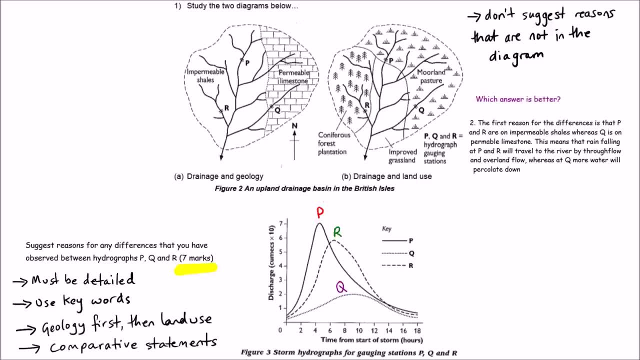 Whereas at Q, More water will percolate down into the rock and travel to the river via groundwater flow, Which is much slower. This explains why Q has a much lower peak discharge and a longer lag time. By using the phrase the first reason, they've given their answer a clear structure. 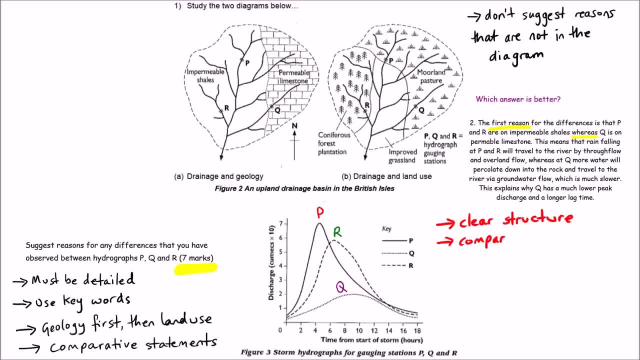 And they've used words from the question. Secondly, they've used comparatives. They've used comparative words such as: whereas They have clearly developed the points they're making by using the phrase. this means that You can see that they've used lots of key words in their answer. 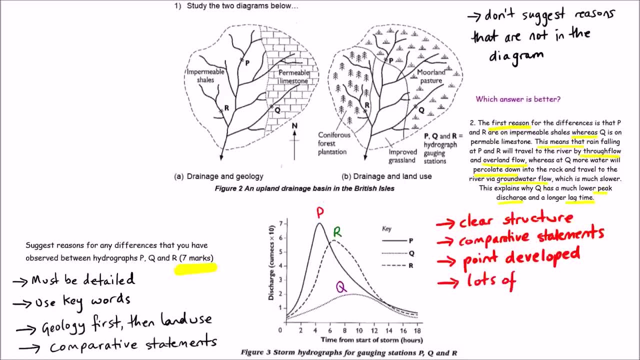 Such as through flow, overland flow, groundwater flow, percolate. They've fitted lots in just to one paragraph And they've also used specific information from the diagram. They haven't made any assumptions. Now, that's only part of an answer. 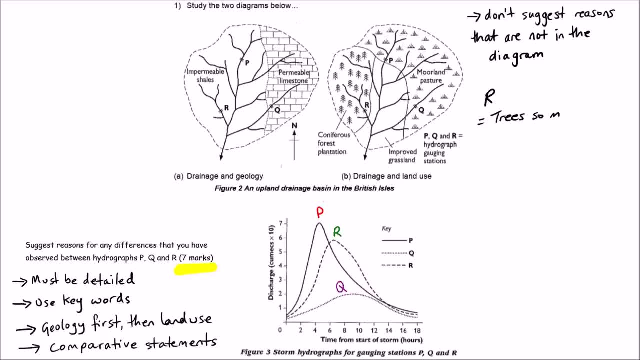 So let's see what else we could look at Now. if we look at R first, R is situated in a coniferous forest, So there's trees which intercept a lot more rain than grass or pasture, for example. This would do two things. 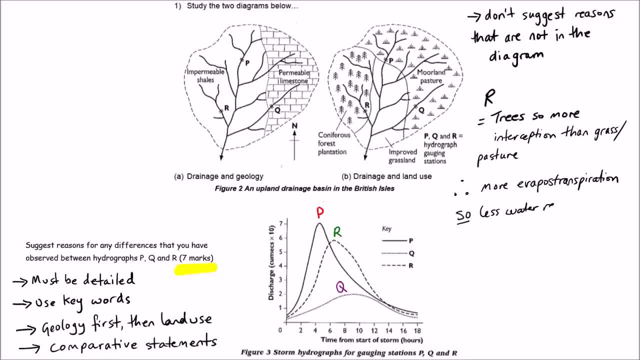 First of all, there would be more evapotranspiration, So less water would reach the river in the first place. This would explain the lower peak discharge. Secondly, This means there would be more sediment. This means there would be more stem flow and through fall. 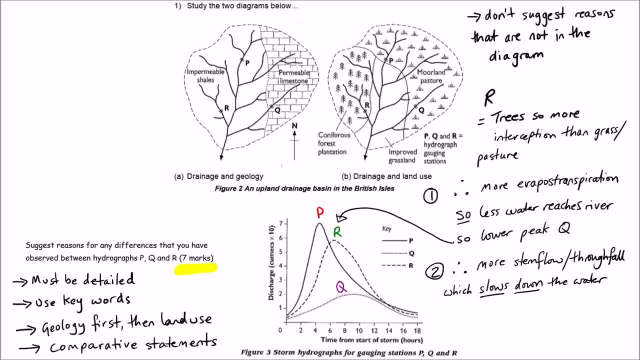 Now this is much slower than if it just falls on bare ground. This would slow down the water and create a longer lag time. Now let's look at Q. You can see from the diagram that it has only one tributary leading into it. 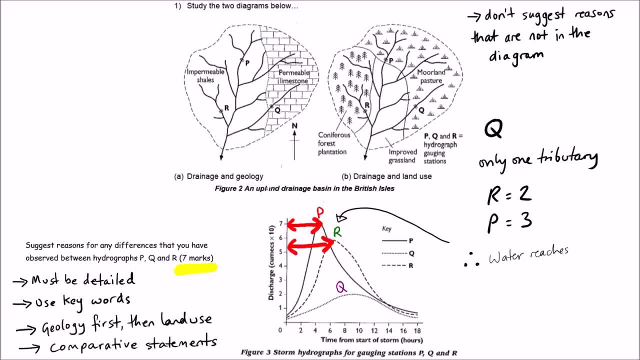 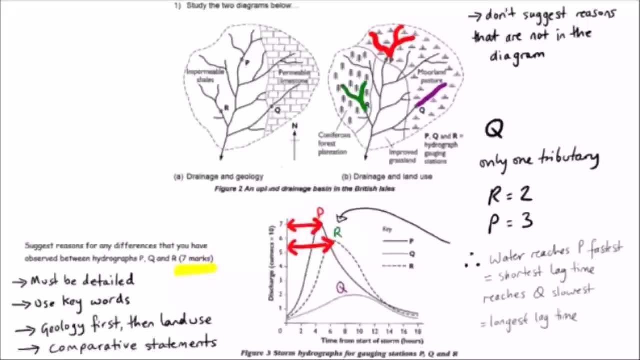 R has two, whereas P has three. So it would make sense that water reaches P the fastest And therefore P has the shortest lag time. And the water reaches Q the slowest And so Q has the longest lag time. So you can see on the diagram here there's three tributaries for P. 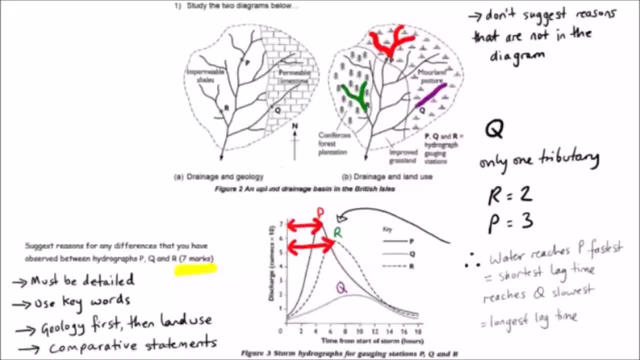 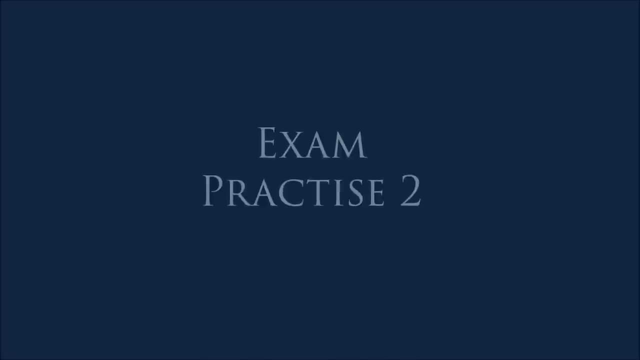 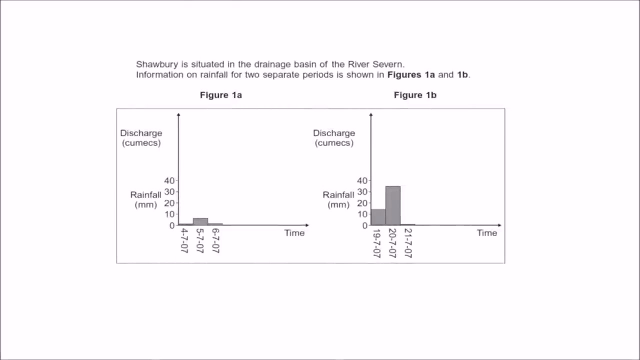 Two for R and one for Q. Now I'm not going to go into any more explanations that you could give from the diagram, But I hope these examples have given you a good idea of how to reach level 2 in this question. OK, so let's look at one final question, which involves practising your graphical skills and drawing hydrographs. 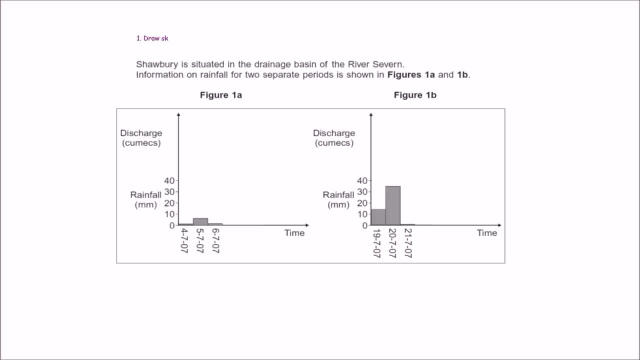 The question says that you need to draw sketch hydrographs on figures 1a and 1b to show the contrasting effects of each of the two rainfall periods on river discharge, And this question is worth three marks. Now, the first thing to remember is that the hydrograph is a line graph. 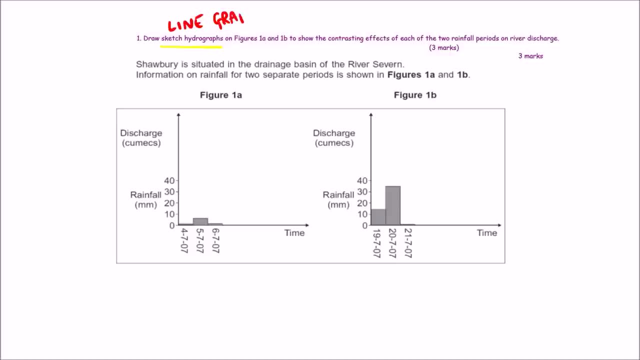 So you don't need to be adding any more bars onto the diagram. Now, if we have a look at the question, we can see that the two graphs are from the same river. It's just that they show different periods. It's not two different rivers, which a lot of people think are the same. 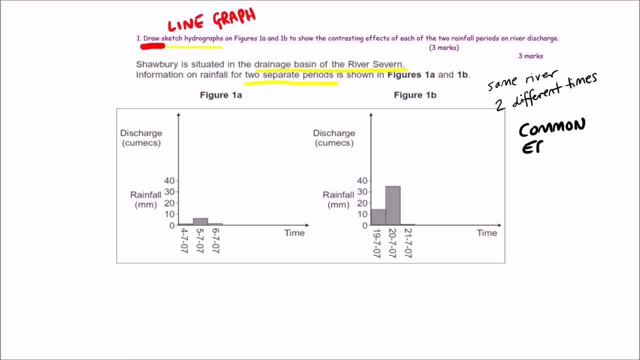 It's just that they show different periods at the beginning and then get confused about. Some of the common errors that people encounter when answering this question is: firstly, they don't give the river any lag time. They don't give the water any time to reach the river. 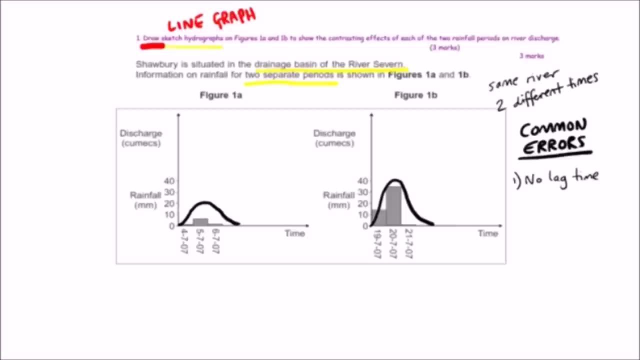 So they draw something like this. So as soon as it rains, the river levels go up instantly, And we already talked about why this is not the case. The second mistake people make is that their river dries up, So by this I mean that they start and end their hydrograph all the way at zero. 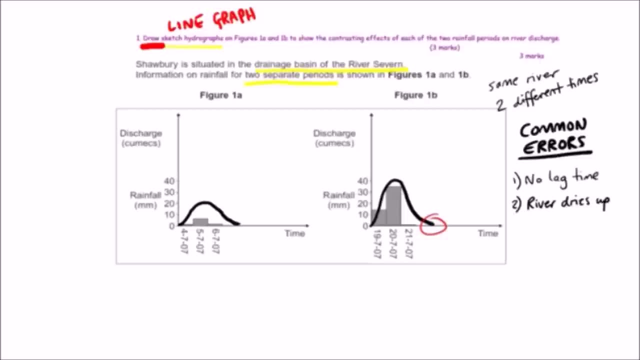 This indicates that there's no water at all in their river in between rainfall periods. Now, while this might happen in a desert, remember that this is the River Severn in the UK, So that's very unlikely to happen. The third issue is inaccuracy. 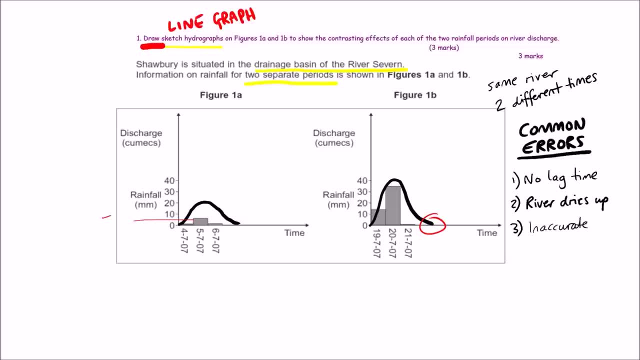 Now you can see in figure 1a the peak rainfall is around 5mm compared to 34mm for figure 1b, So evidently there's a lot more rain in figure 1b. Therefore, there should be a lot more discharge in the river. 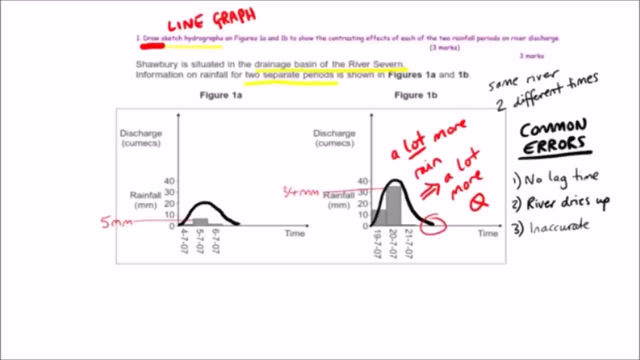 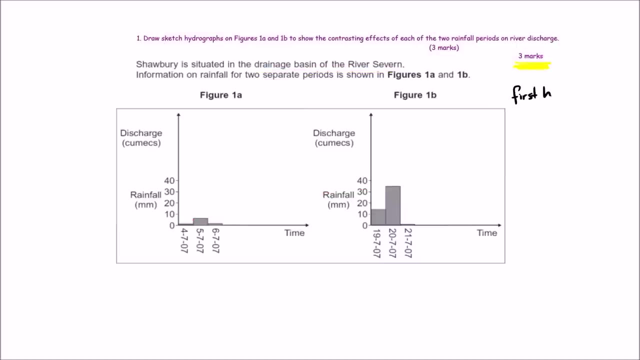 Unlike in this sketch, where the second hydrograph isn't really that much bigger than the first. So how can you get your three marks for this question? Well, firstly, the hydrographs have to be correct overall, So let's draw them on. Now you can see that I've started and ended both hydrographs. 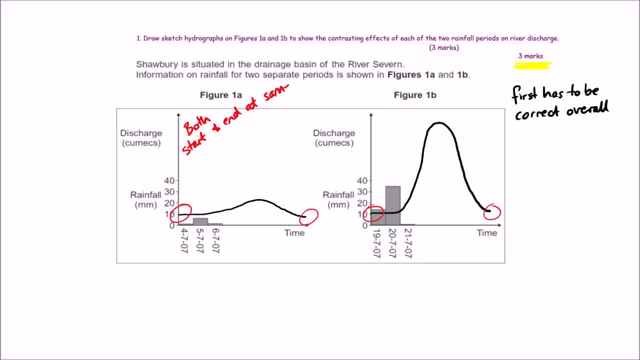 at the same level Because, remember, both hydrographs are the same river, So it makes sense that they would start and end around the same level. Secondly, I've made sure that my peak discharge is after my peak rainfall, So I've given them some lag time. 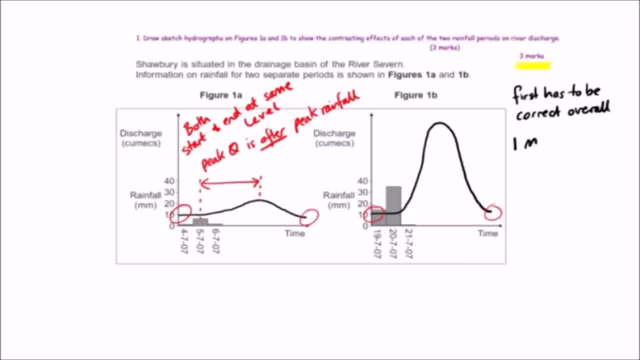 If they go down to zero, you can't get more than two marks. So once you've got them correct overall, you can get one mark. for making sure that your second hydrograph has a higher peak discharge than your first hydrograph, You can get a second mark. 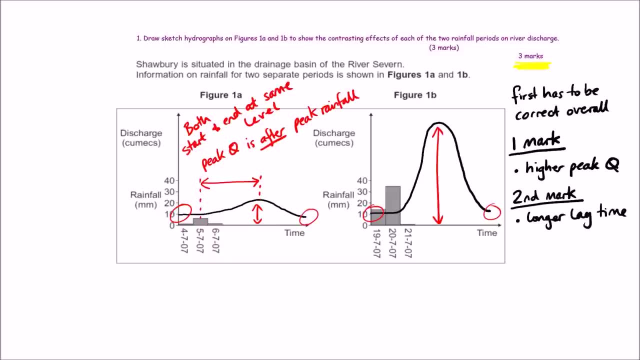 for making sure that the first hydrograph has a longer lag time than the second. And then, finally, your third mark would be for accuracy. So the peak discharge for the second hydrograph needs to be at least three times as high as the first one. 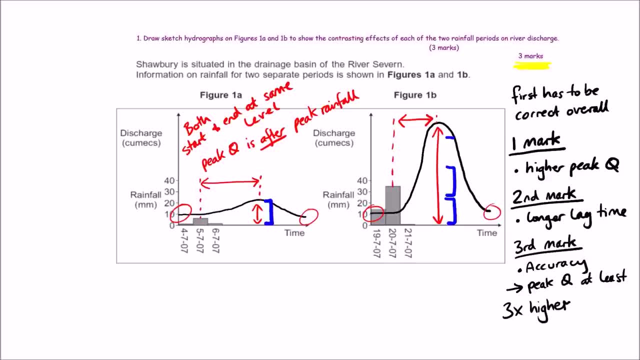 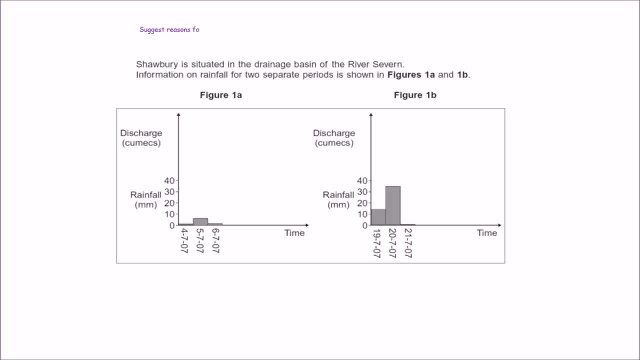 And that's because the peak rainfall on the second hydrograph is so much higher than the first. Now for the second half of this question. you have to suggest reasons for the differences in the shapes of the hydrographs that you have drawn. Now this is worth three marks, which means it's point marked. 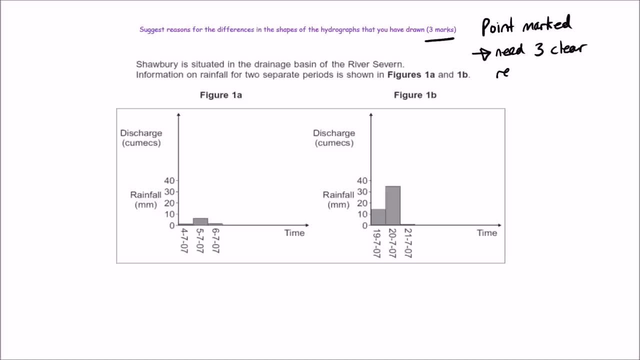 In other words, you need to give three clear reasons for three points, And you must explicitly link these reasons to the hydrographs that you've drawn. So let's draw our hydrographs on again Now. you can structure your answer by firstly, describing the shape of each hydrograph. 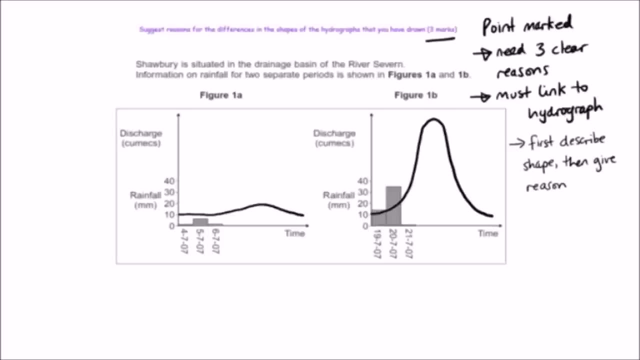 And then you can give a reason why it's that shape. So, for example, you could say that 1a has a longer lag time because peak rainfall didn't even reach 10mm, meaning that most of the water would have infiltrated into the soil. 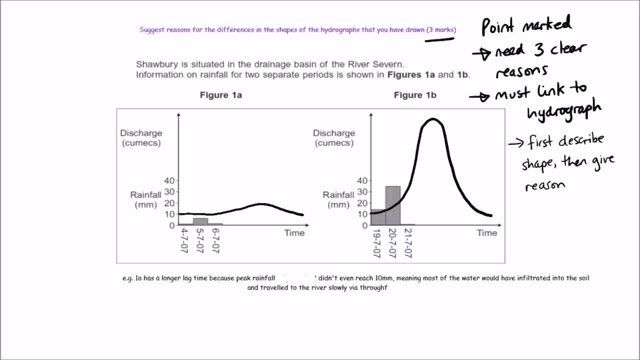 and travelled to the river slowly via throughflow and groundwater flow. However, 1b has a shorter lag time because it gets a lot more rainfall- over three times as much. This would saturate the soil, leading to overland flow which would reach the river.